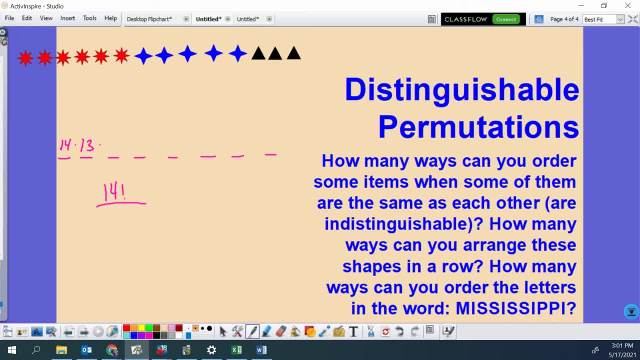 separately in your 14 factorial figure. so that doesn't tell the whole story, but that is a good starting point. you know, if, if we had a little marking on each one of those objects, then that would be right. right like if, if this was like red star one. 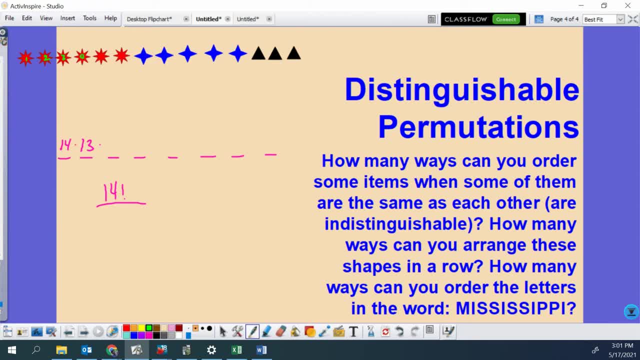 red star two, like if there's a little number on each one to make them look unique, right, um, that's sort of like a little barcode or something, right, um? or maybe i wouldn't call that. seven and eight, maybe this would be. blue star number one through five, right? 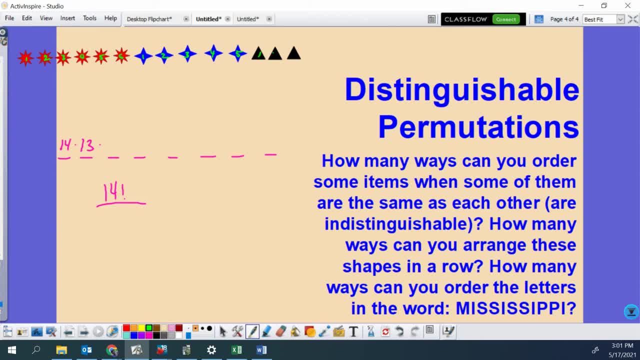 if we had that, then the 14 factorial would tell the whole story. right, that would be right. um, however, we don't, and we want to count all the red stars the same and all the blue stars the same and the three black triangles the same as well. uh, let me just point out before we get into. 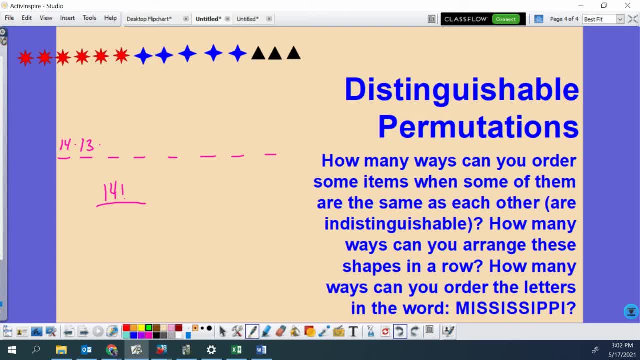 how to, how to hone in on those distinguishable permutations, how to remove the indistinguishable repetitions? uh, before we hone in on that, let me point out what that 14 factorial is. so 14 factorial. let me use a better color there. 14 factorial is 14, p 14.. how many ways can i do a permutation of 14 objects out of 14 objects? that's what that. 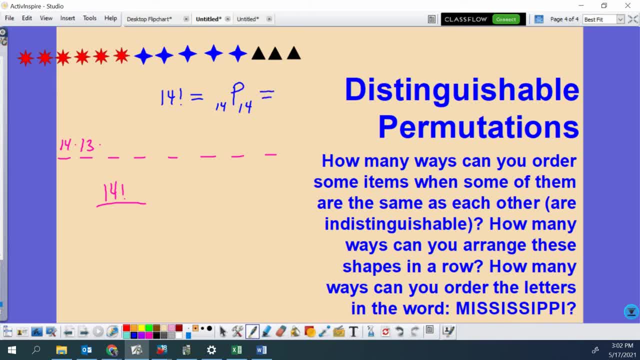 means and the formula for permutations. um well, npr. whoops, and you saw this in the last video. if you watched, that is uh n factorial over n minus r factorial. so in this case, with 14 p 14, it would be 14 factorial over 14 minus 14 factorial. and if you're looking at that, scratching your 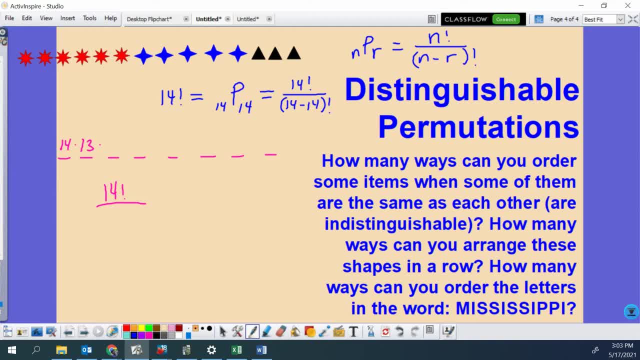 head like: wait a minute, what's going on in the denominator there? you should know- uh, it's important to know this for combinatorics in particular- that zero factorial is one that's important. if you're wondering why, um well, the best reason is that it kind of needs to be a. 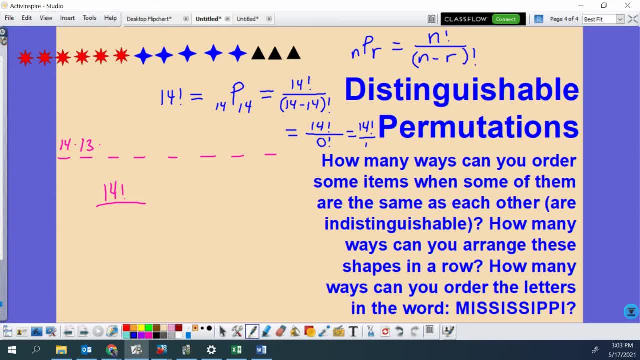 in order for combinatorics to work, So that when you take the number of ways that you can do a combination of five things out of five things, if you plug it into the formula it doesn't work, if that's zero right. 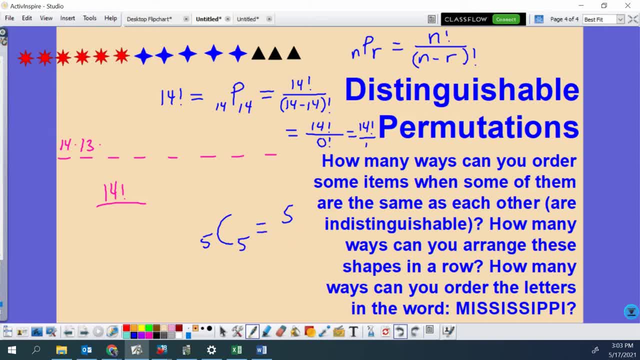 That's my best answer. We could dive more into that maybe another time, but for this video we'll just leave it at that. Zero factorial is one that's important to know, Anyway. so 14P14 tells you how many ways. 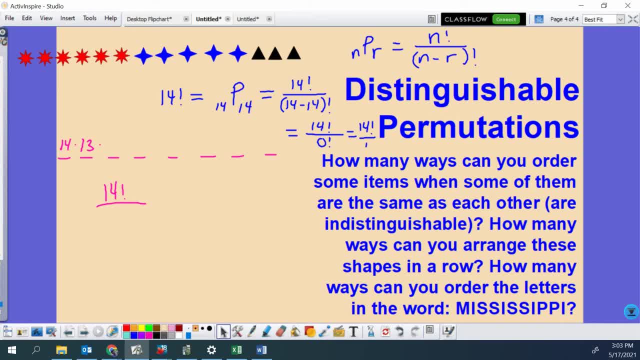 you could order 14 different items. The problem is that in this case, we don't have 14 different items. In this case, we have 14 items, but six of them are one thing and five of them are another thing, and three of them are another thing. 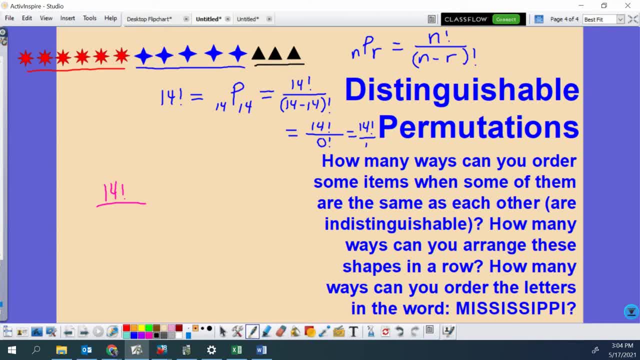 And so what you need to do now is think: okay, once you pick one of these arrangements, right, Once you pick like the one I have up here, right? Or let's shift it around a little just to mix it up. 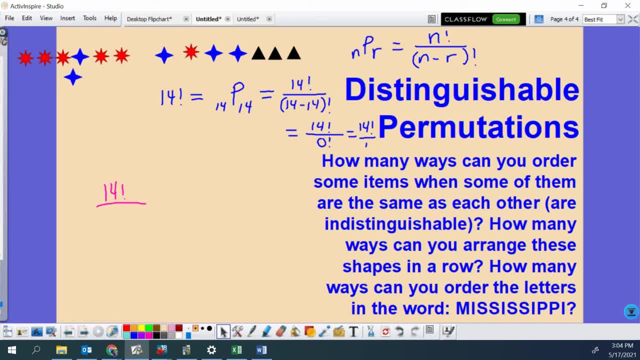 Once you pick- that was a silly one to move. Once you pick one of these arrangements, maybe this arrangement right here. let's make it a little more interesting. The question is, how many times does that arrangement get counted in the 14 factorial? 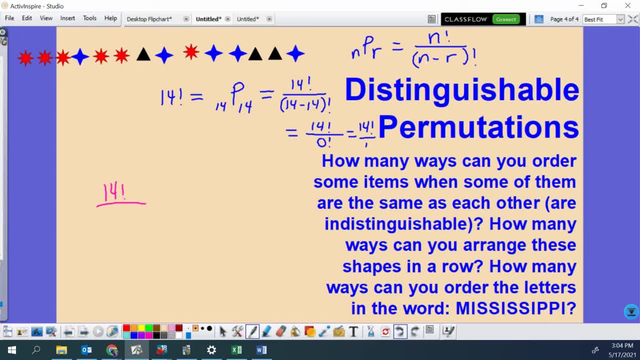 How many repetitions, how many duplications do we have, right? How many redundancies? And so what you need to realize is that within each shape, there's a bunch of repetitions, right? For example, I have five blue stars: One, two, three, four, five. 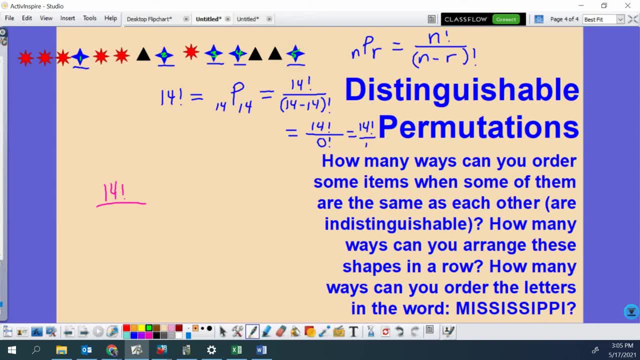 I had them numbered earlier, right, And what I could do is I could reorder those, I could switch one and two, and if that's all I do, that's another one of these 14 factorial ways to do it. So the question is, how many different ways do I? 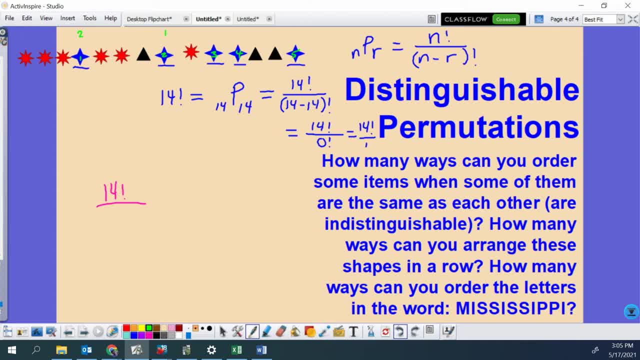 can I order those five blue stars? really right? That's, if we can do that, then we can take out all of the five blue star duplications that are in this 14 factorial. And so if you ask yourself, how many ways can I order these five blue stars? 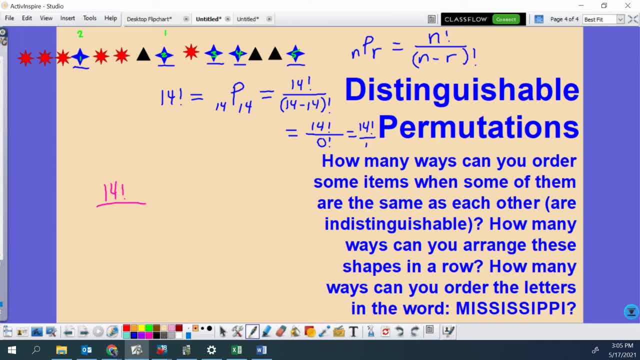 It becomes a much simpler problem. right, There are five blue stars. Whatever order, whatever organization we have, whatever solution, whatever distinguishable permutation, I guess, is what I want to say there is, there are going to be five blue stars in it. 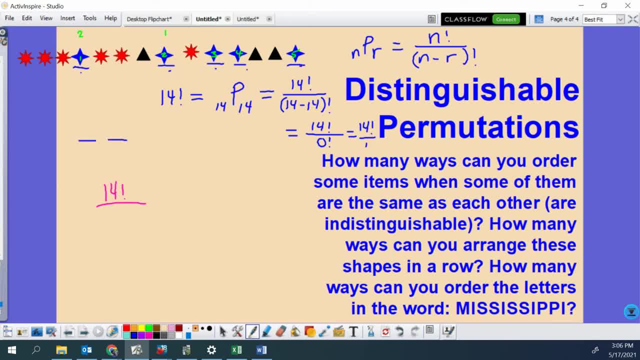 And if you just focus on those and ignore everything else- one, two, three, four, five- you have five slots now. And what do you have? You have five choices for the first slot, right, It could be star. one, two, three, four or five. 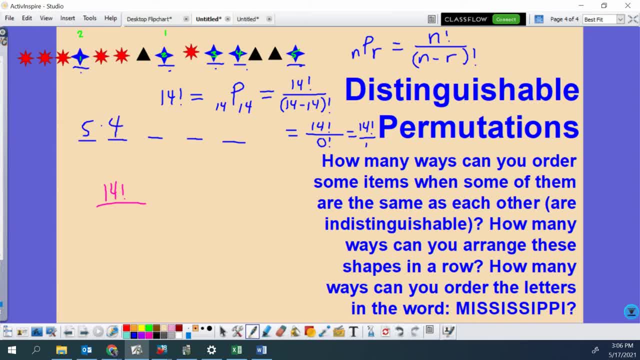 And then, once you pick one, you have four and then three, and then two and then one. So it's really five P, five or five factorial ways to arrange the five blue stars, And for each one of those five factorial equals 120 ways that you can arrange those five blue stars. 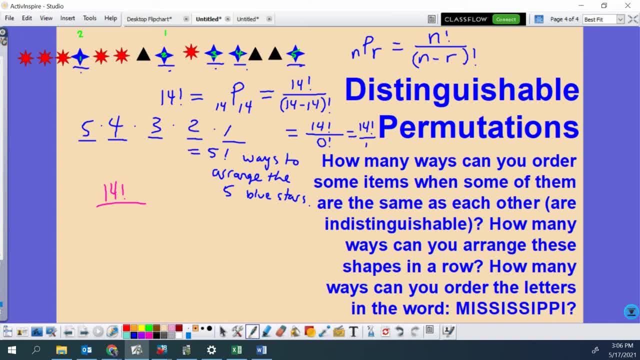 for each one. we counted all of them in the 14 factorial. but we don't want to. They're all the same to us, because we don't see those little green numbers on the blue stars. We just see the blue stars. And so because of that, 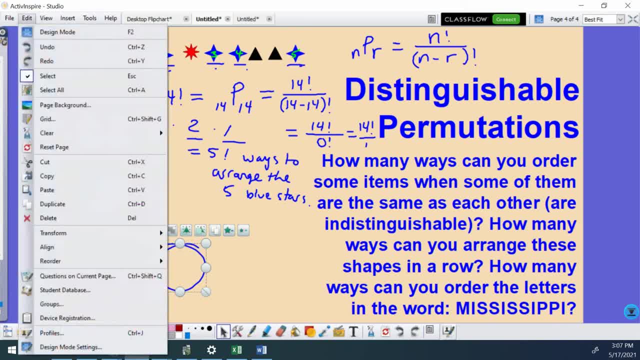 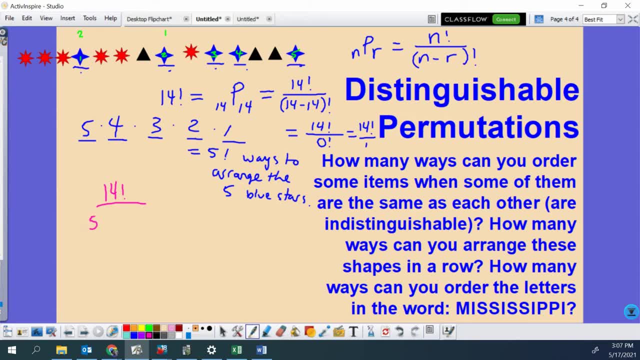 what we really want to do is we want to divide that out. We want to divide out the five factorial to remove the repetitions from the blue stars. Okay, And we're going to do the same thing then with the red stars, right? How many red stars are there? 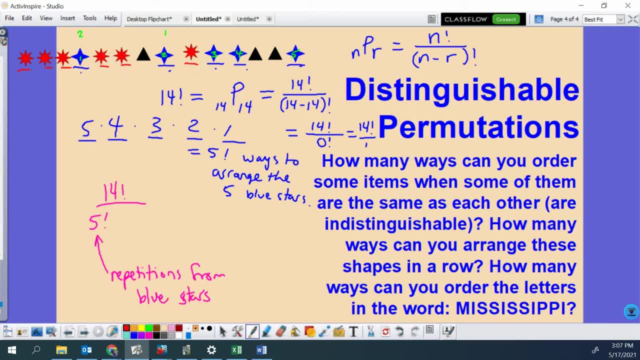 One, two, three, four, five, six. They're indistinguishable. I could number those one to six and then I could distinguish them Every single ordering, of those six red stars, of which there are six factorial right. 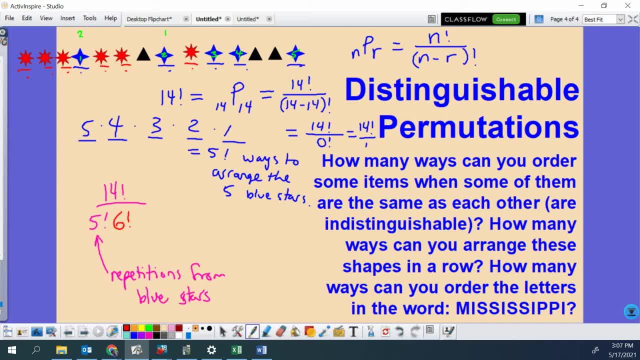 Let me do that in the same color there. Well, no, let's leave it. I like that. In fact, let's make the five factorial blue to match the blue stars. Every single ordering of those six red stars is represented in the original 14 factorial. 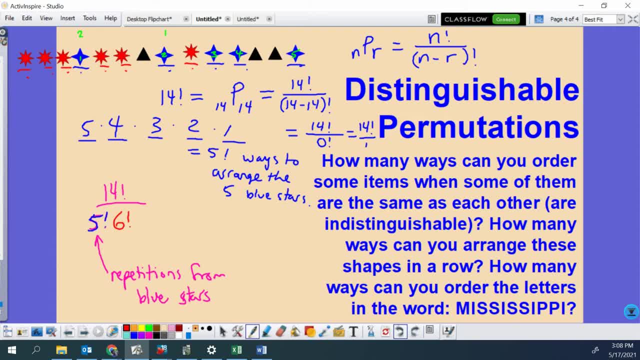 And there are six factorial ways to order the red blue stars. Just like there were five factorial ways to order the five factorial The five blue stars, I think I said red blue stars, The six red stars is what I meant to say, And so we need to divide all those out also. 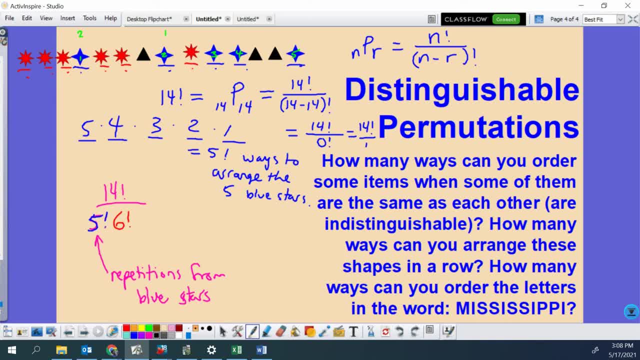 Those are all repetitions, right? And then we're going to do the same thing for the three black triangles. We're going to divide out a three factorial And we just divide all of them out. Those things are all multiplied together on the bottom. 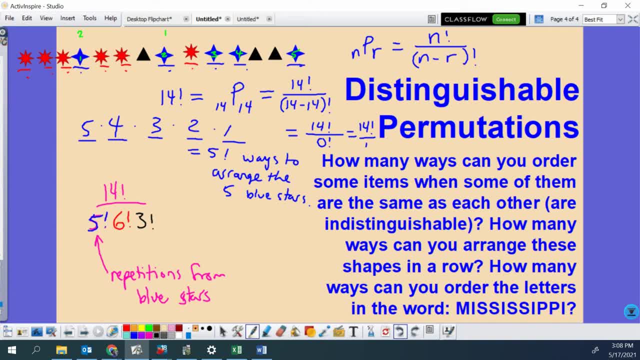 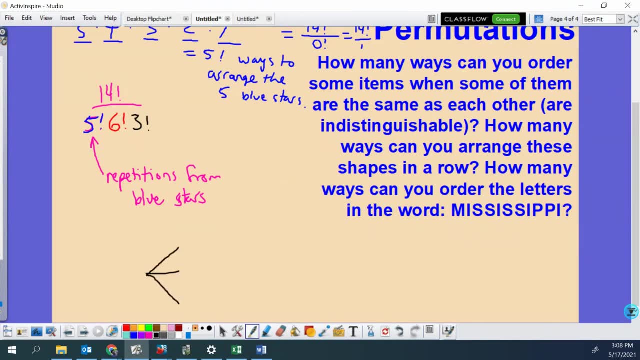 In fact, you could kind of picture a gigantic- and it would be enormous, an enormous tree diagram representing all the different combinations of those repetitions, Right? So, like, how many different ways can you arrange the three black triangles? Well, you have three branches on that tree, right? 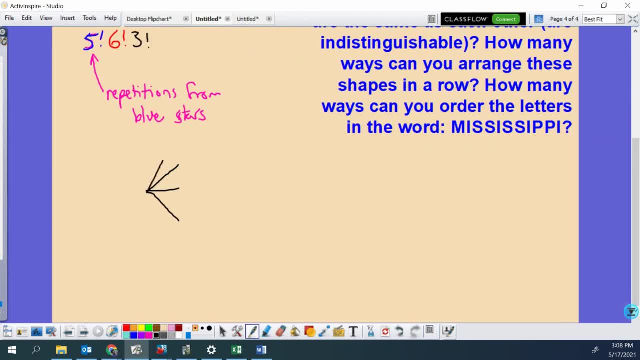 You could. I'm sorry, You have three factorial. You have six branches on that tree right, You could do triangle one, triangle two, triangle three, triangle one, triangle three, triangle two, triangle two, triangle one, three, two, three, one. 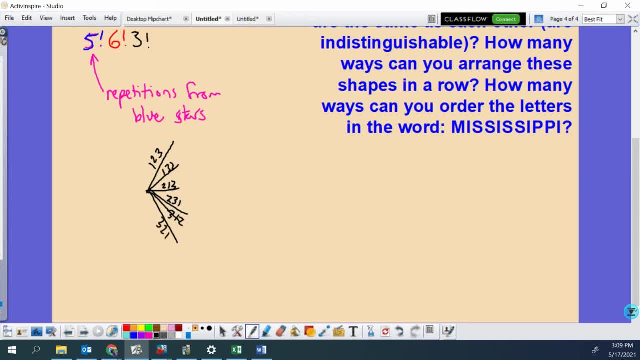 and then three, one, two, and then three, two, one. Those are all the different orderings, So you could have a three partial orderings of the three black triangles. That was the easy one. Now for the blue stars. 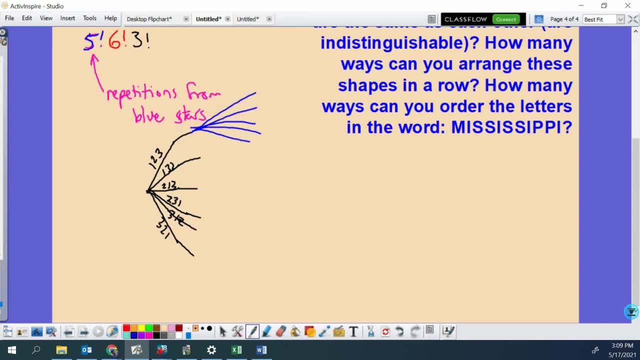 there's five factorial different orderings. That's 120.. So I would now need 120 blue branches in my tree diagram off of each one of these. I need 120 of those to show all of the different orderings of stars, one through five. 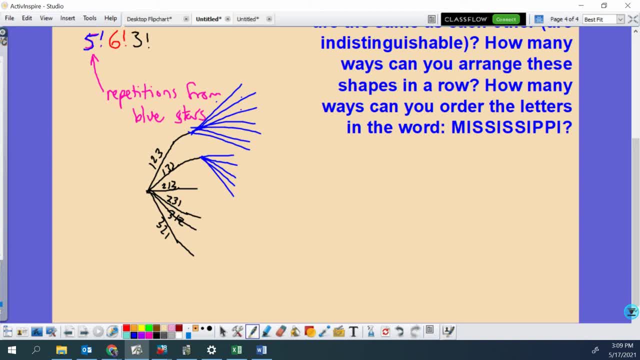 So I would have like one, two, three, four, five, One, two, three, five, four, And you know, and so on, and so on and so on. of those branches I would need six factorial, which is 720 branches in red, coming off of all. 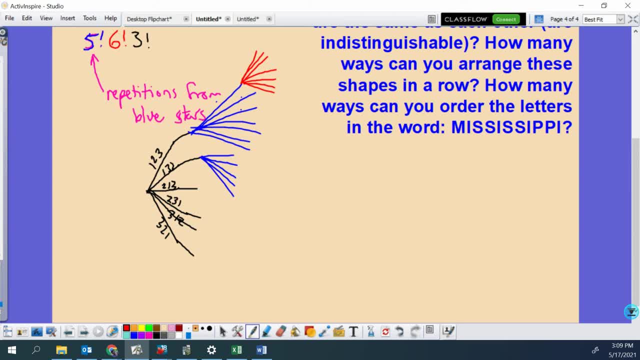 of those 120 times six branches in blue, And so it ends up, I think, being 720 squared, because three factorial is six, which makes that like another six factorial. Anyway, it's a lot, right, There's a big number in that denominator. And those are all of the repetitions, because 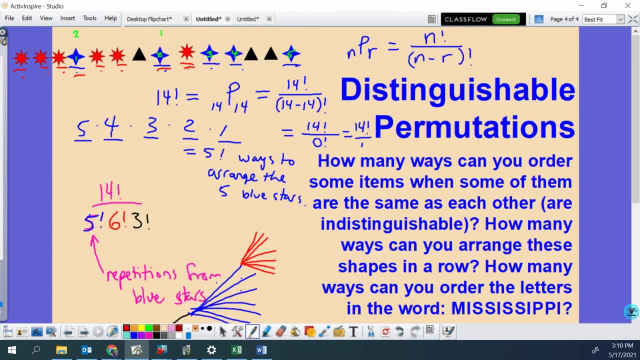 for every ordering you can do of the blue stars. you can also combine that with any one of the orderings for the red stars and any one of the orderings of the black triangles, And so those multiplied together are really the total number of repetitions of indistinguishable 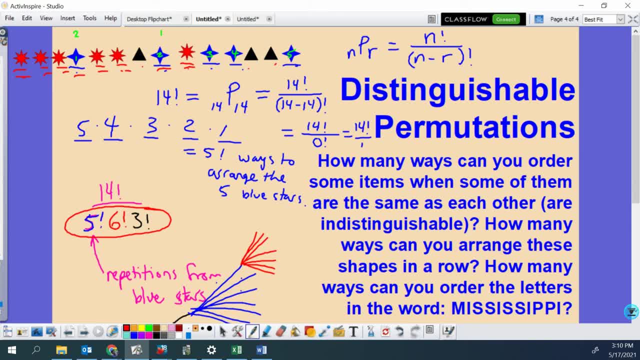 I'm sorry- of distinguishable permutations, right, The number of times we repeat each distinguishable permutation. if we just do five, 14 factorial. So that's really the formula If you want to find the number of distinguishable permutations of n items and you have x1 of item 1 and x2 of item 2, and so on. dot, dot, dot. 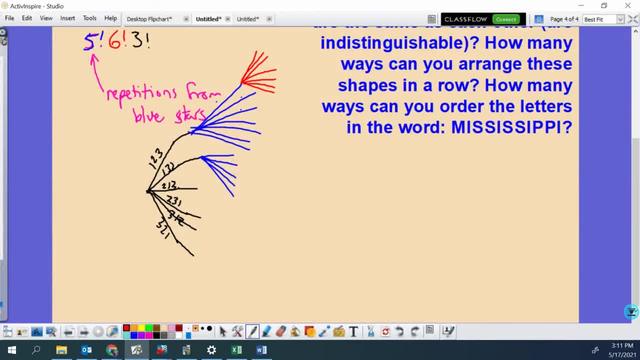 the formula that we're going to have is going to be n- factorial over x1 factorial times, x2 factorial times. you know, dot, dot, dot, until you get to x, I'll just say k- factorial. if there are k different items, total And that's. 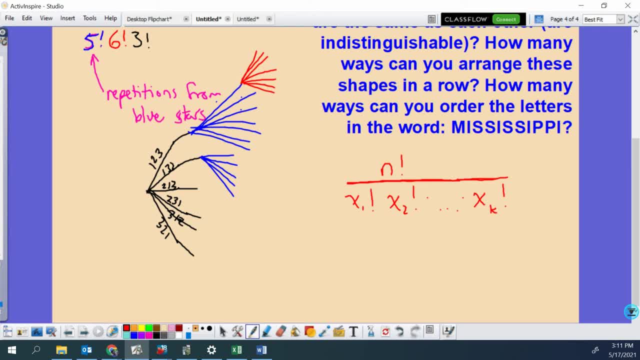 it. It's a pretty simple formula to use, but that's why it works. Hopefully that makes sense. Let's look at one more example really quickly here: The word Mississippi. If you rearrange letters in the word Mississippi, just make them all caps so we can't tell the difference. 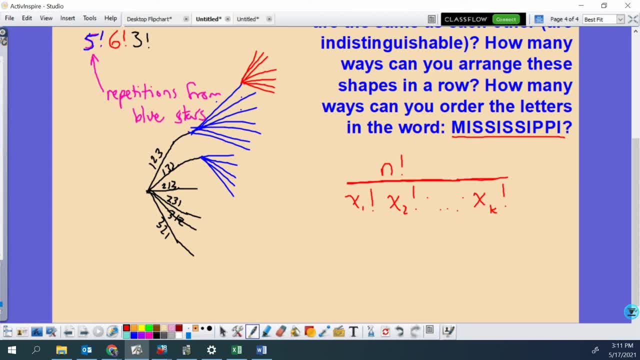 between any of them. The question mark is not part of this question, And so it might be worthwhile to count each letter. We've got four S's, We've got four I's, We've got an M And we've got two P's. I think I counted that right. What's that? 11 letters, 1,, 2,. 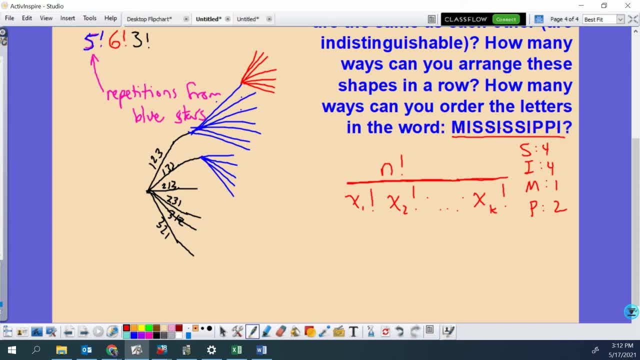 3, 4,, 5,, 6,, 7,, 8,, 9,, 10, 11.. Looks good to me. So how many ways can you rearrange those that are different from each other? Well, there's 11 factorial ways to rearrange 11 letters, But within that I have rearranged. 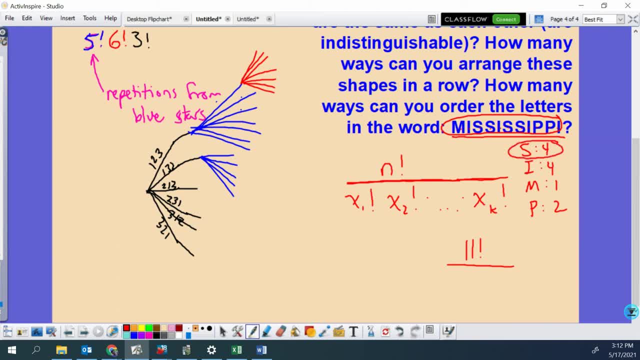 my S's, S1 through S4, and I've counted all those arrangements. There are four factorial of those arrangements. I have to divide that out. Same thing with the I's. I have to divide that out. You can put a one factorial in here for the M, but you don't need to because there's only one. 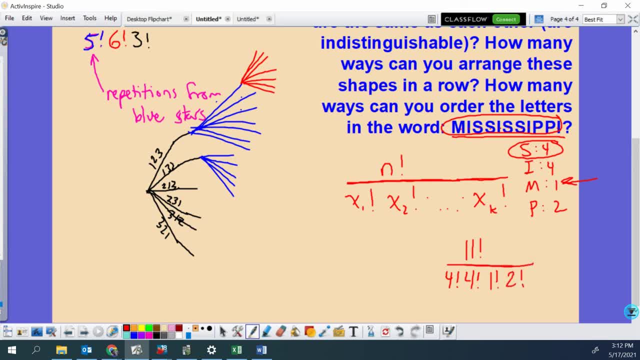 of them. So you can put a one factorial in here for the M- but you don't need to, because there's- and then two factorial for the P, And then, while you're at it, you could even throw in a zero factorial for the zero Q's in the word Mississippi, And it won't affect the answer, because remember. 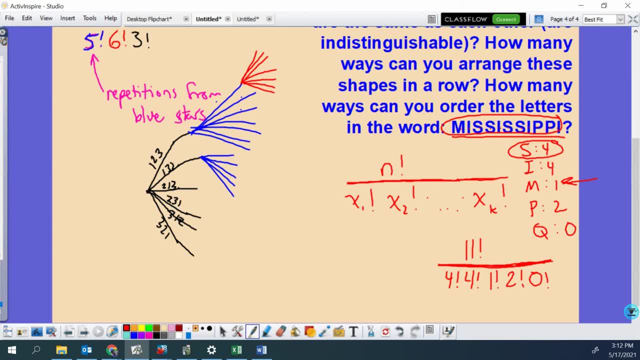 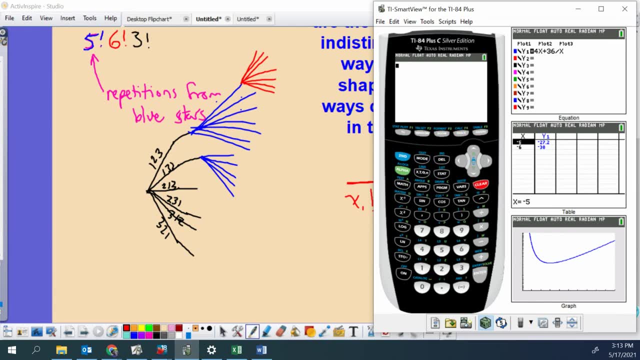 zero factorial is one. I just thought I'd throw that in there again. I didn't bother to actually compute these. I guess I could. I have a graphic calculator right here, And if we wanted Mississippi, let's do that one. I want to say alpha, Where's my? 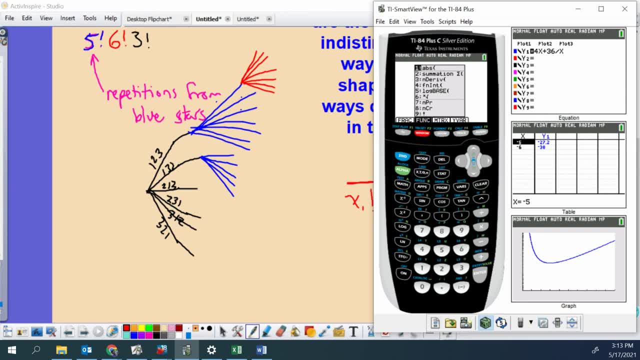 Oh, that's not the right one Function. Oh, there we go. Yeah, Factorial is choice nine here. So let me get back out of here. I want a fraction and I want 11 factorial on top, Choice nine. And then I 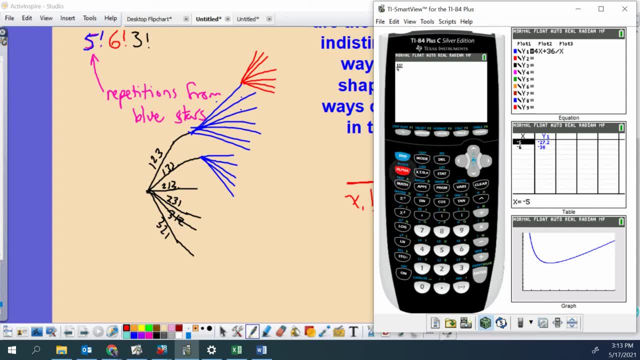 need a four factorial, a couple of those, Another one And a two factorial. I'm just going to put times two, because two factorial is two And there are 34,650 different ways you can rearrange the letters of the word Mississippi and have them actually. 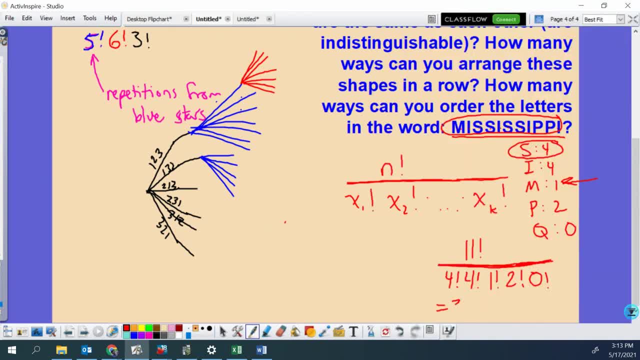 look different: 34,650.. The numbers can get pretty big because you're dealing with big numbers when you have factorials. If you want to do something like this by hand, if you're taking a math competition and you're not allowed to do it, you can do it by hand. You can do it by hand. You can. 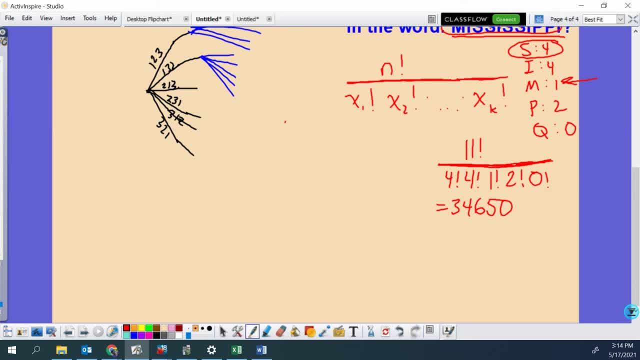 use a calculator, You might think, hey, that's absurd. How could I do that by hand? They're not that bad, though. Factorials are actually kind of fun to work with by hand. What I would do on this: 11 times 10,, nine, eight, I get down to four, seven, six, five And then I just do a four. 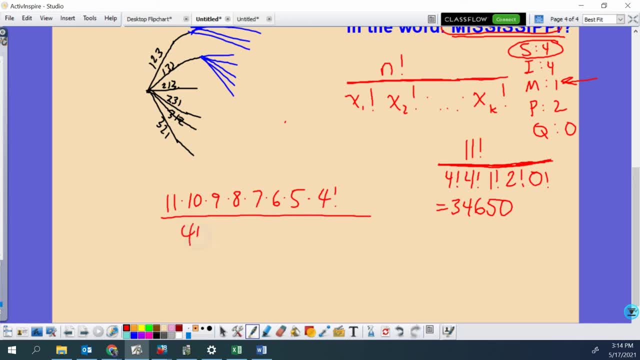 factorial. And then we got four factorial, four factorial and two factorial, And then start canceling stuff And you can cancel a lot. typically Four factorial is four times three times two. So if stuff doesn't match up quite right, I might just do four times three times two. leave out the 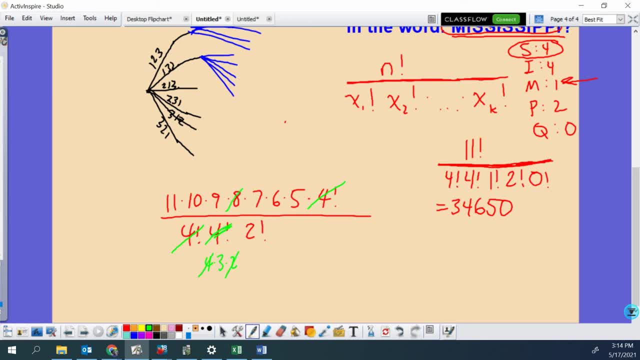 one, And then you can reduce the four and the two with the eight, And then you can reduce that three and that two with the six, And you end up with 11 times 10 times nine times seven times five, which is a little less daunting. I'm not going to have you watch me multiply that out. 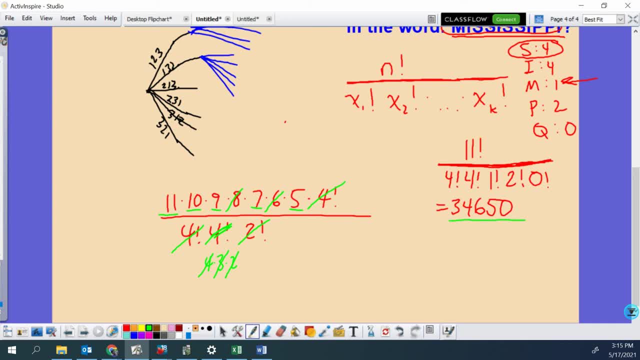 but we could probably all get through that one without too much pain. Anyway, that's all there is to distinguishable permutations. It's kind of like when you're dividing out the those factorials on the bottom. It's a lot like when you take permutations and you divide out.